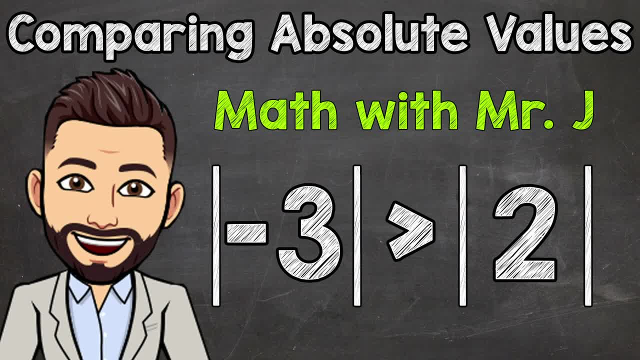 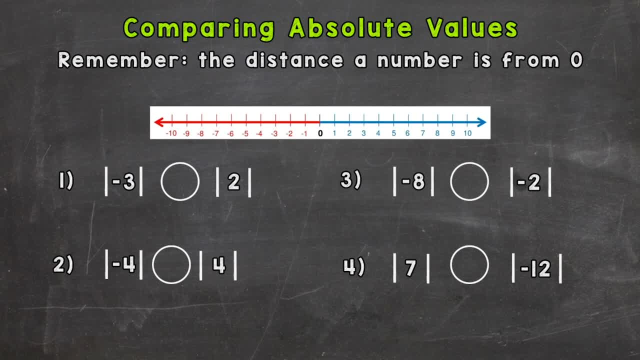 Welcome to Math with Mr J. In this video we're going to take a look at comparing absolute values and remember the absolute value is the distance a number is from zero and if you take a look at your screen, we have four comparisons that we're going to go through together in order to get this. 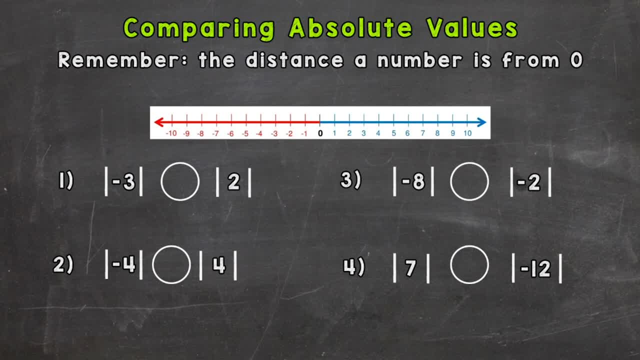 down. So let's take a look at number one and get started, and we have the absolute value of negative three compared to the absolute value of two. So let's use the number line for this one in order to help us visualize which one's greater. So let's do the absolute value of negative three first. 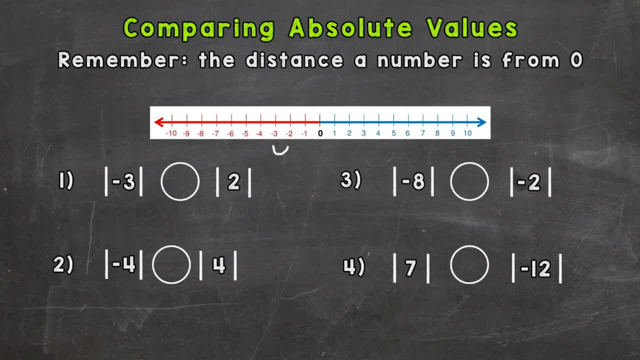 So negative three is one. two three has a distance of three away from zero, So I'm going to write the absolute value of negative three underneath. It has an absolute value of three. That's how far away it is from zero. Now a positive two is well. 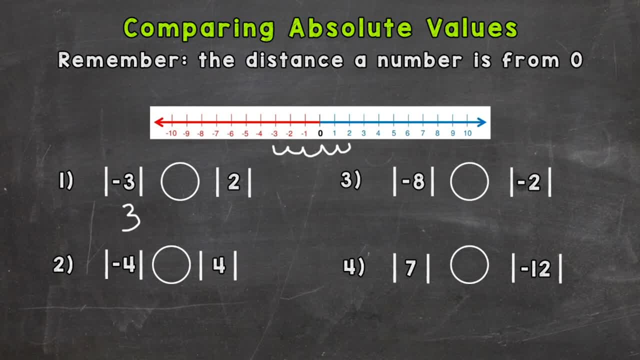 one. two. It has an absolute value of two. That's how far away it is from zero. So now that we have the absolute values written, we're able to compute the absolute value of negative three. So let's go ahead and compare, So which one has a greater distance from zero? Well, negative three has a. 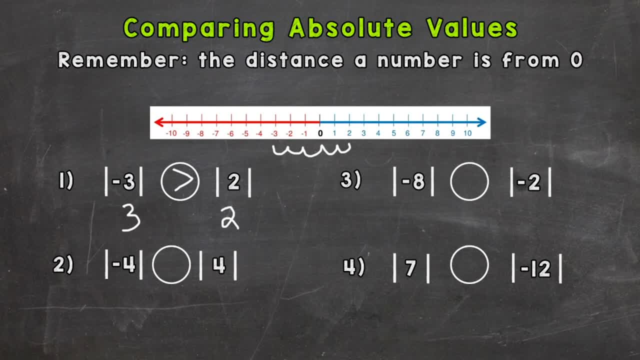 greater absolute value. So we can read that from left to right: The absolute value of negative three is greater than the absolute value of two. Now, if we were just to compare negative three and a positive two, well, the positive two would be greater, But since this is absolute value and the 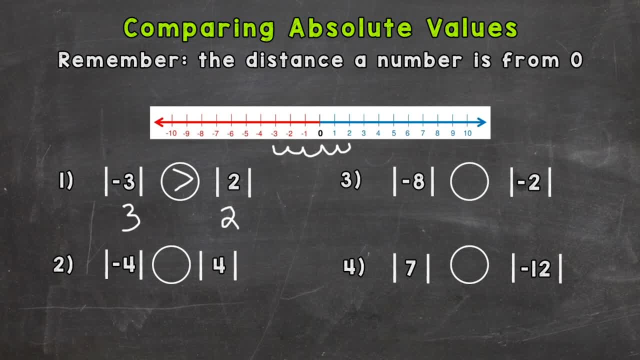 absolute value is площ uma over two. we can multiply the value of negative three by two. Now again, because of the fact that we have that line and the distance from zero, that negative three, the absolute value of negative three is greater. So let's take a look at number two, The absolute value of negative four. 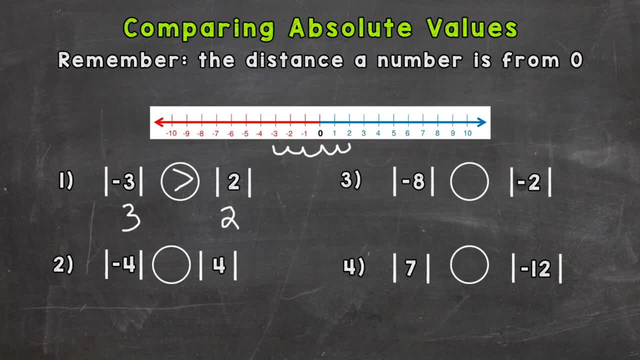 compared to the absolute value of four. Well, let's write the absolute value of both of those below. that way we can compare. So the distance of negative four from zero, That's the distance away, or the absolute value of negative 4, is 4.. 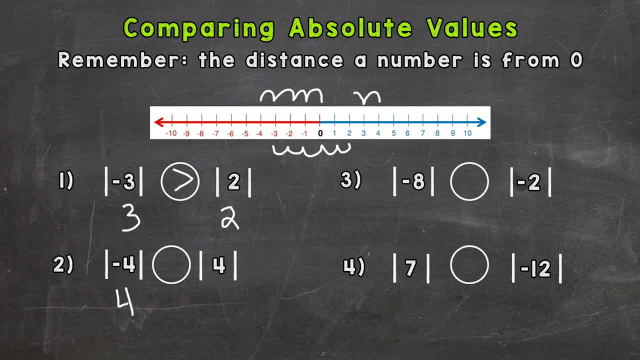 Let's do positive 4.. 1,, 2,, 3, 4.. So positive 4 also has an absolute value of 4, the distance from 0. So the absolute value of negative 4 is equal to the absolute value of a positive 4.. 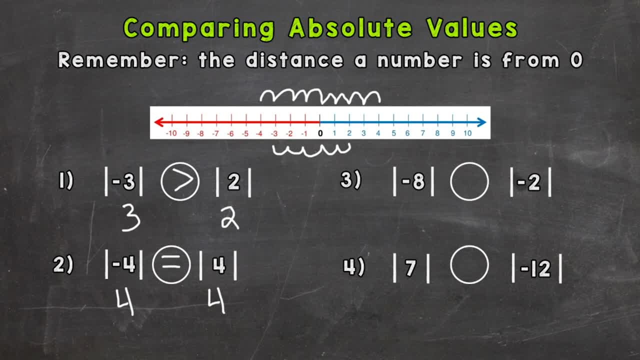 They both have the same distance from 0.. Let's take a look at number 3.. So we have negative 8, or, I'm sorry, the absolute value of negative 8 compared to the absolute value of negative 2.. Well, the absolute value of negative 8, or the distance from 0, is 8.. 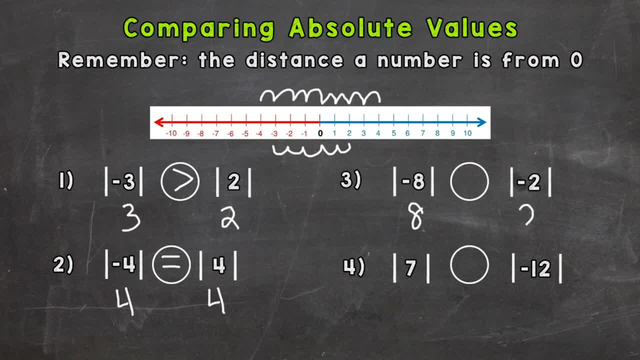 And the absolute value of negative 2 is 2.. So for this one the absolute value of negative 2 is 2.. So negative 8 is greater than the absolute value of negative 2, right: Negative 8 is a further distance from 0 than negative 2.. 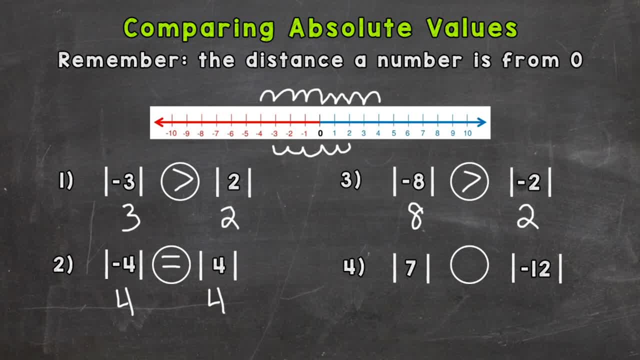 And, lastly, we have the absolute value of 7 compared to the absolute value of negative 12.. Well, the absolute value of 7 is 7, the distance from 0. And the absolute value of negative 12, or distance from 0, is: 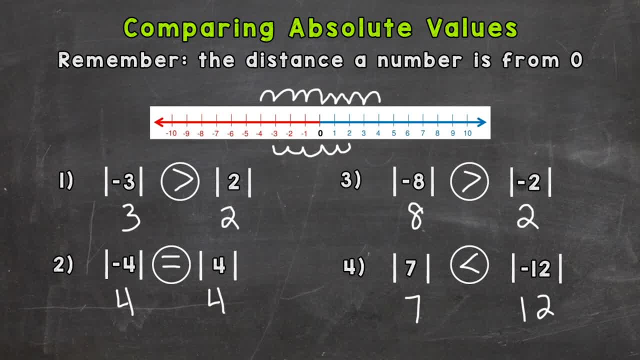 12.. So here we have: the absolute value of 7 is less than the absolute value of negative 12.. Now, if this was just a positive 7 compared to a negative 12 there, and absolute value was not involved, that 7 would be greater. 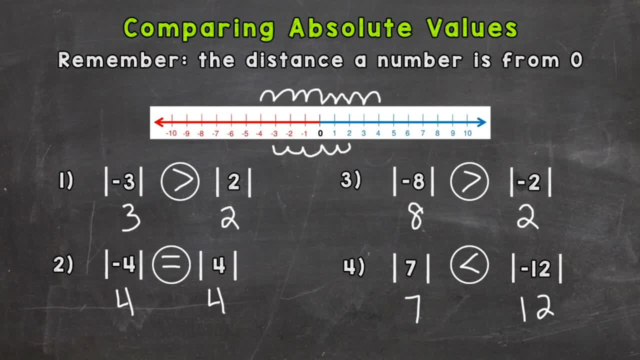 But since it's absolute value- and you're just taking a look at the distance from 0, that negative 12, the absolute value of negative 12 is greater. Hopefully that helped. Thanks so much for watching. Until next time, peace.